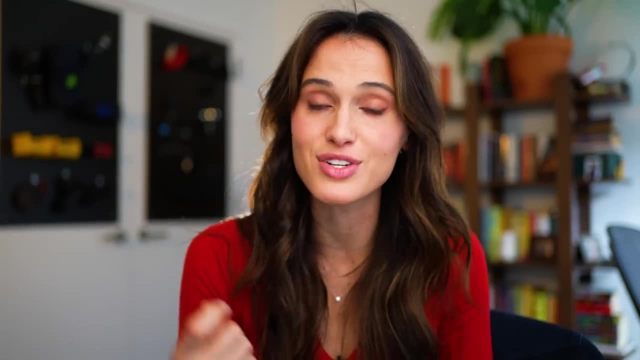 There's something totally different, and that difference is actually the key to understanding why they're such a big deal, Why governments around the world are using computers in a more correct way And those who accept them are. I think world are battling it out to build them the fastest. 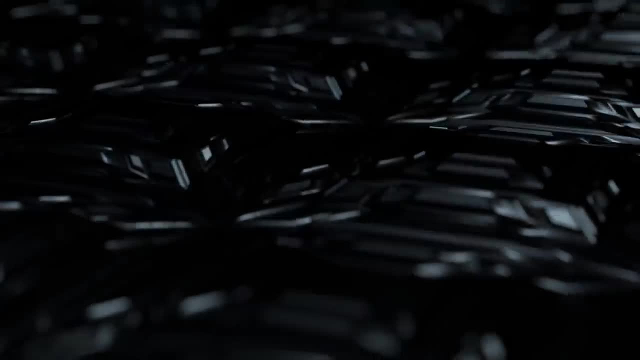 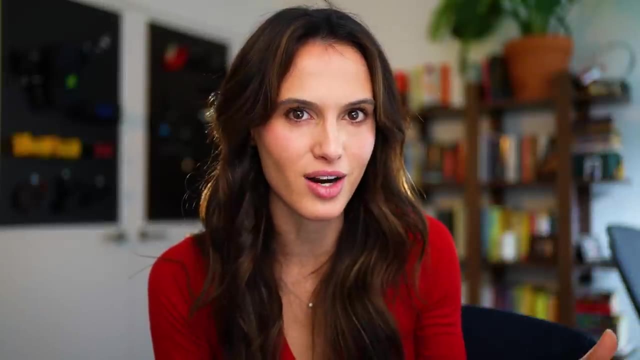 Quantum computers are wild. They're on track to change what we can build and how we understand the world. They're kept at temperatures colder than space. but if you think you really understand how they work, you're probably wrong. At least I didn't. 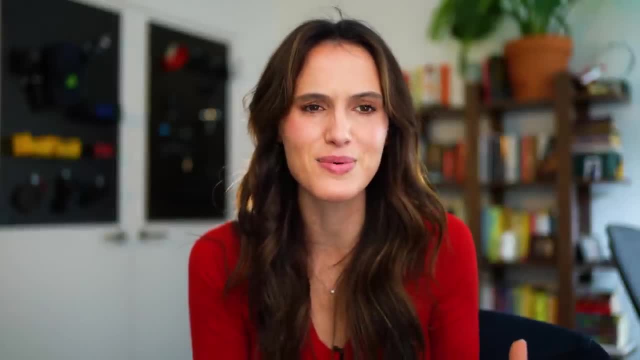 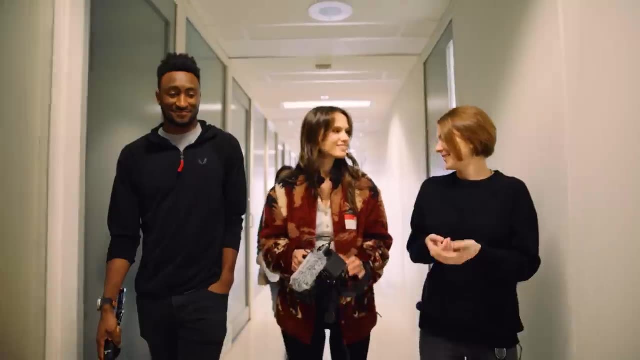 And that's where this video starts. Marques and I both realized that there was this big, important technology that we really didn't understand. So we decided to go on an adventure to figure out the truth about quantum computers, what they can really do and why we should care. 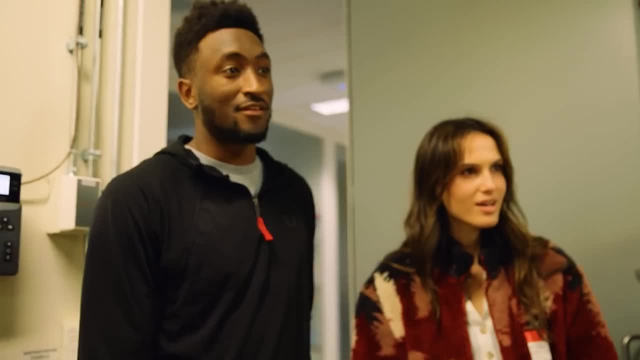 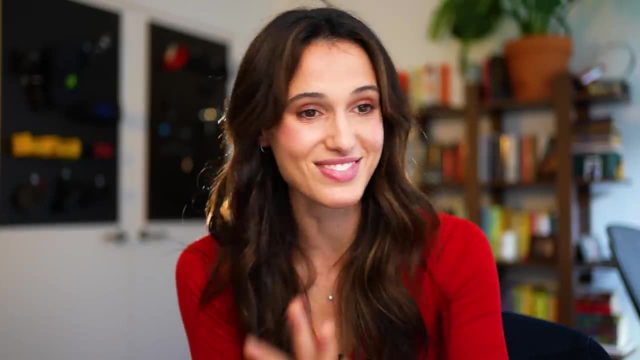 And, of course, we're taking you on that adventure with us, to show you what we learn as we learn it and, more importantly, to show you how these crazy computers might actually impact your life, and sooner than you think. It's a very new skill we just got. 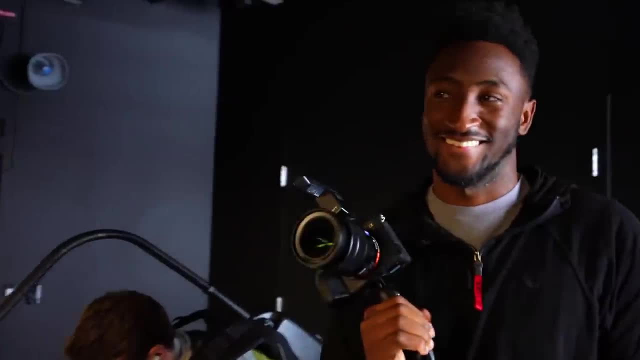 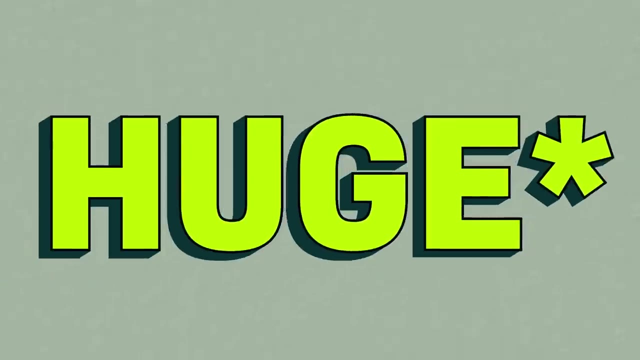 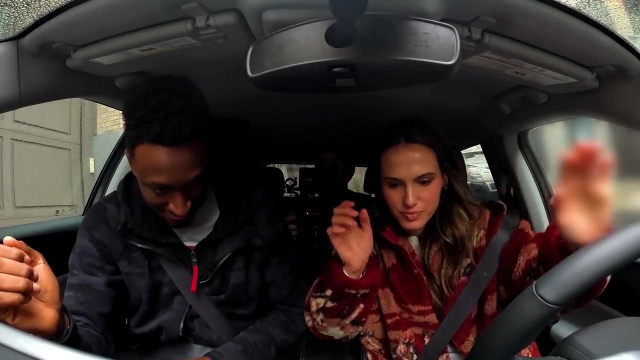 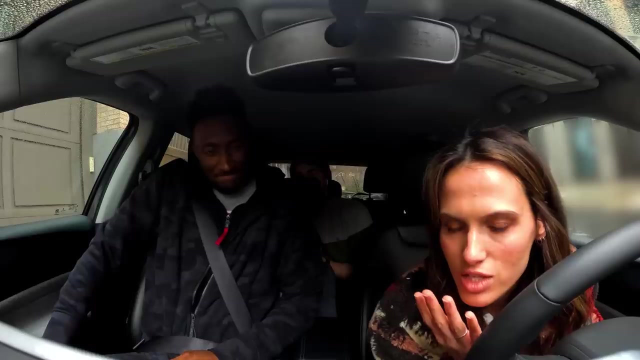 which is being able to hear when a quantum computer is working. What does it sound like? What does that mean? So it works, It's not broken, I swear. I'm usually good with tech, but Like the only function of this screen. 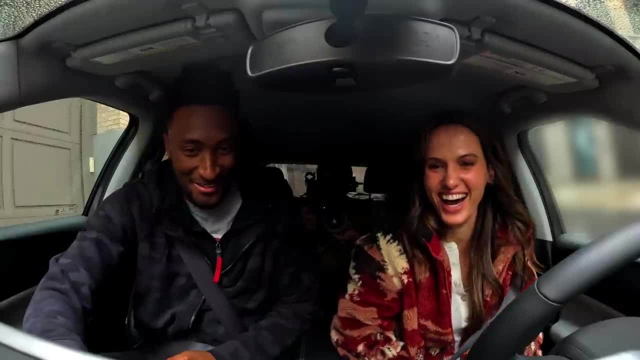 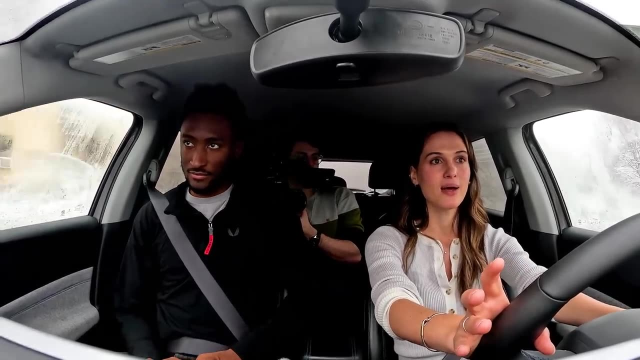 is to provide directions. You're getting this. So we're going to visit IBM's quantum computer. This is really exciting that they're letting us see this computer, because it is, to my knowledge, the largest quantum computer that exists, which I say with confidence. 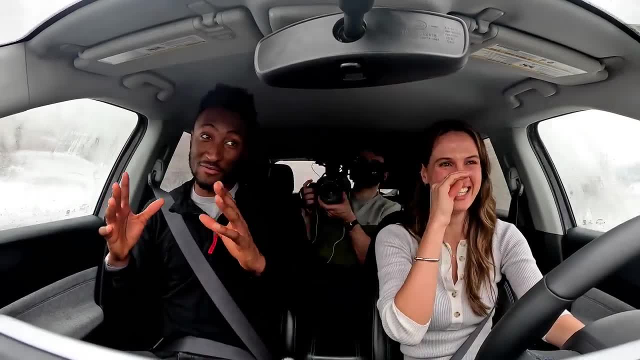 Like I know what that means. I was going to say what is biggest Because, like I heard you know, like supercomputers they're massive rooms full of computers and when someone says we have the biggest supercomputer, 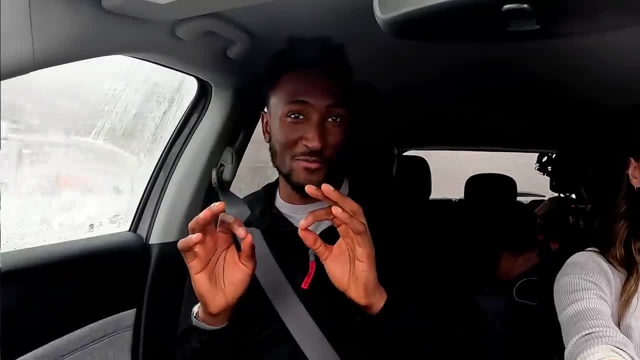 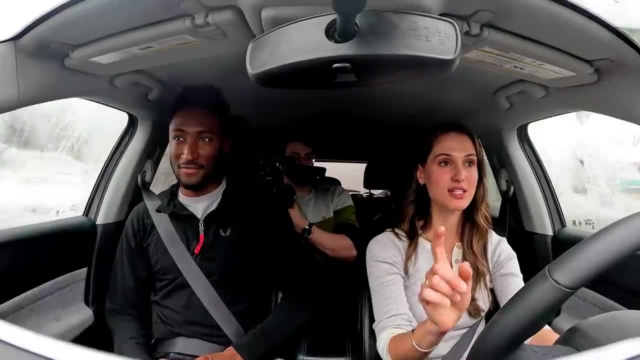 I'm like, oh, I can picture that, The largest quantum computer. I'm not even sure what to picture. I imagine the golden octopus. You know that thing that Biden looked at like this, The press images. yeah, And I know that in order to see that, 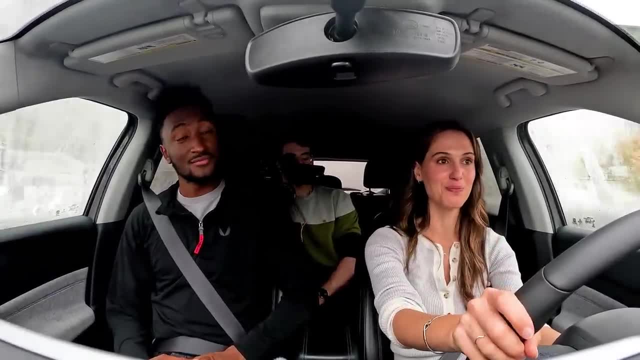 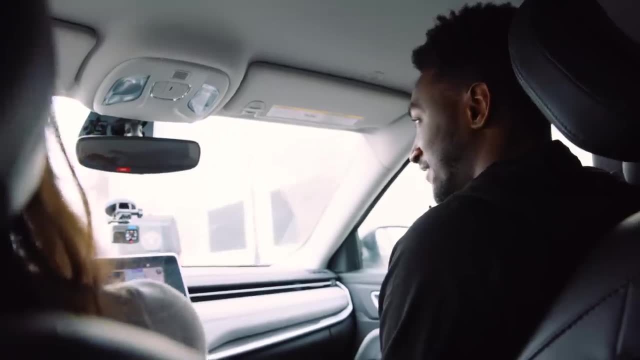 they have to shut down the computer. So this is like took some real logistics on their part. This is a real deal. What is most interesting to you about quantum computing? It's definitely on the edge of my expertise, I would say. 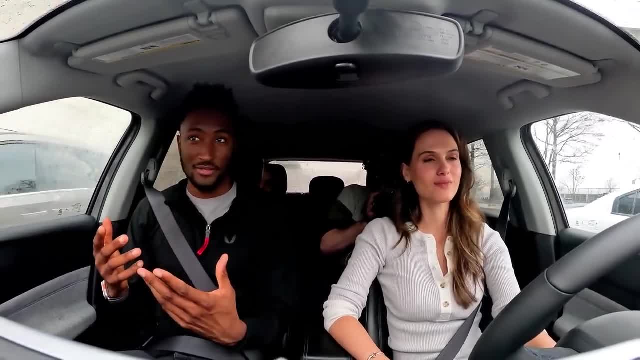 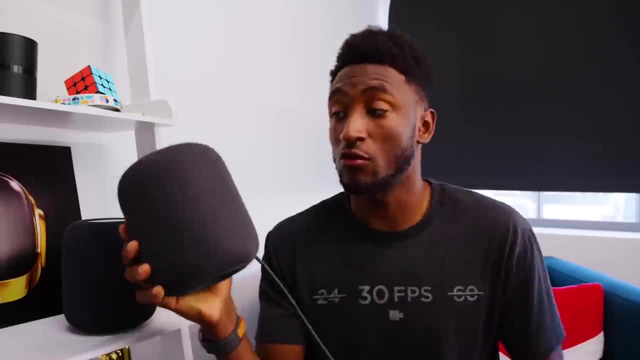 I'm really curious about when it's actually going to touch. like regular people, My whole concern is purchase decisions. At some point in the future, quantum computing will come into play with a real purchase decision. Some will have like a device that they can buy. 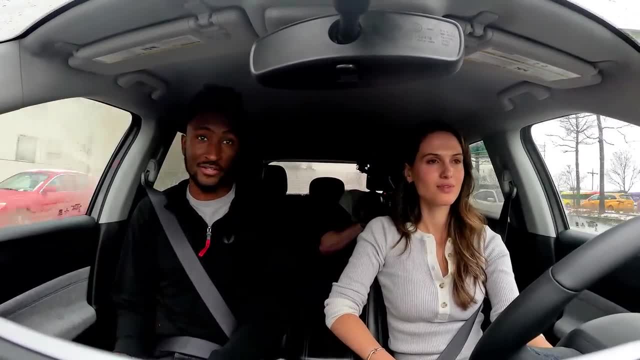 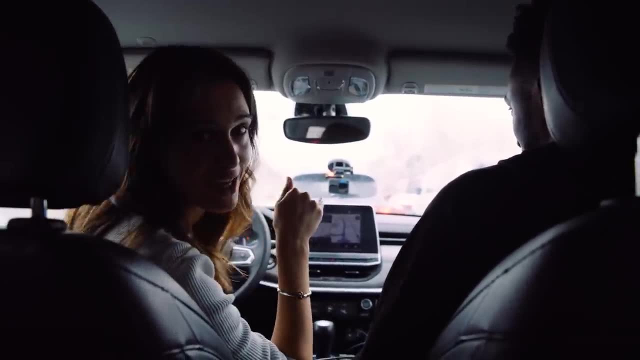 where quantum computing is a part of it or maybe went into its creation at least. When are we going to get to that point? One of the things that I think is very important to make clear is: this is a different kind of explainer. 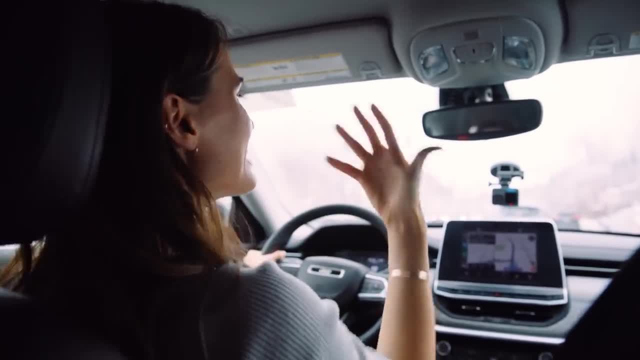 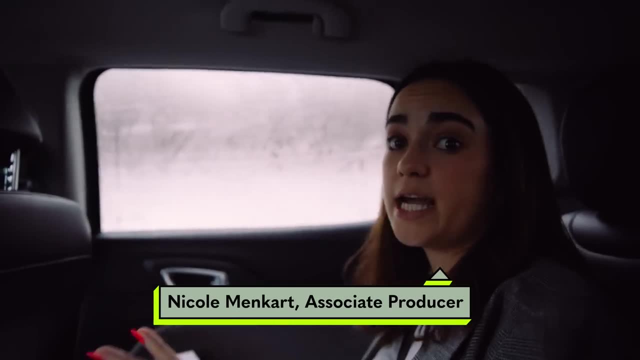 You're just coming with us as we figure this out. Exploratory explainer- Exactly the whole new genre. Along for this adventure are Cody and Nicole. Nicole is an associate producer on this episode who is also studying quantum communication for her PhD. 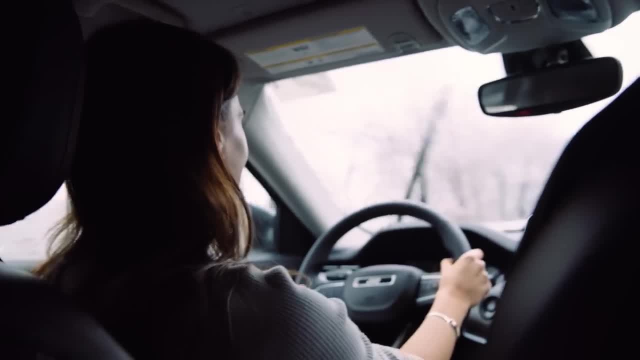 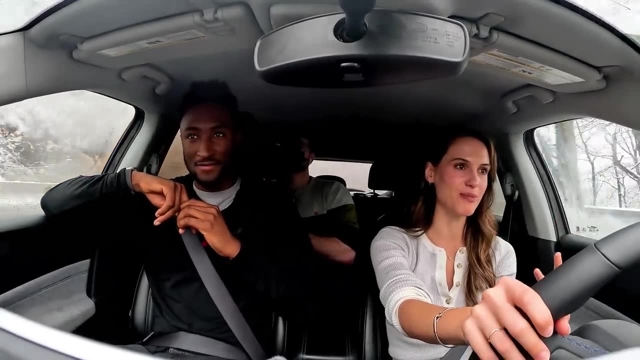 And Cody is our DP, the man behind the camera. Thank god they're both here. So when I started doing this episode, I spoke to a really famous quantum physicist. He was really frustrated at the way that people were talking. They were talking about quantum computers. 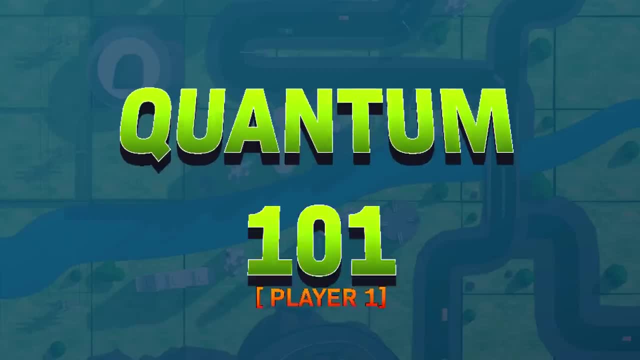 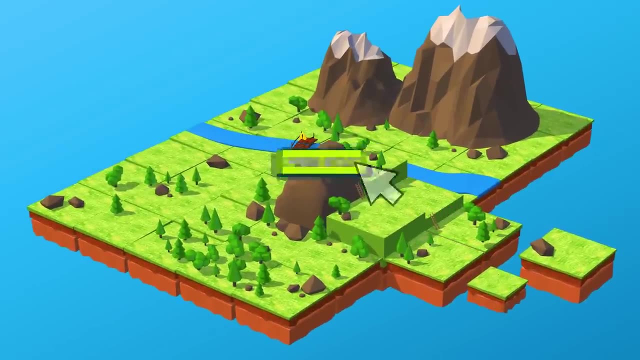 And I was like: OK, how do you want people to think about them? like them? OK, here's the analogy that helps me understand what quantum computers are good for. Imagine that you're on a video game map And how you get around depends on how good. 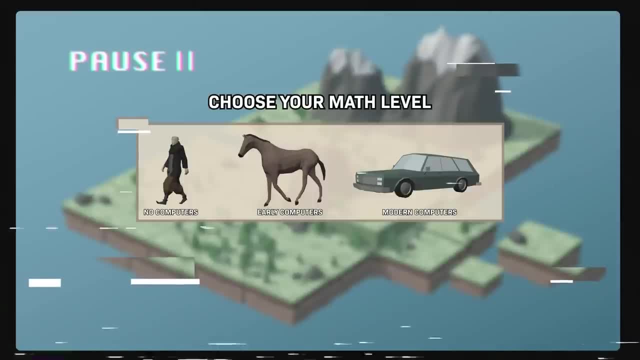 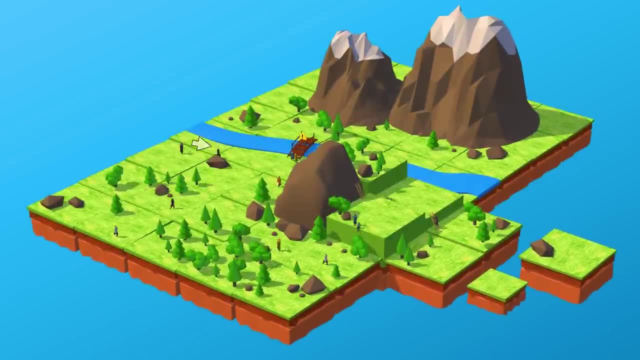 you are at doing math, You may not want to play this video game, Bear with me. So first there were no computers. Things like geometry and astronomy took forever. So you have your little pencil and paper and you're traveling across the mathematical map by walking. 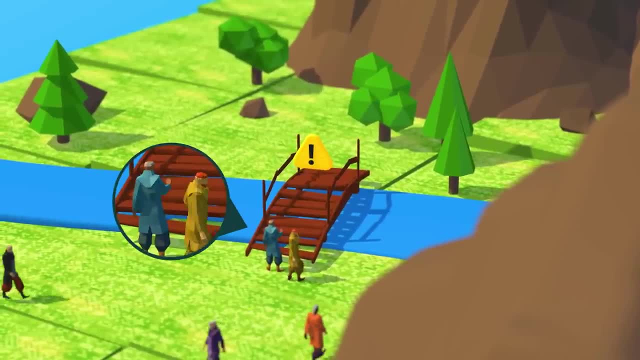 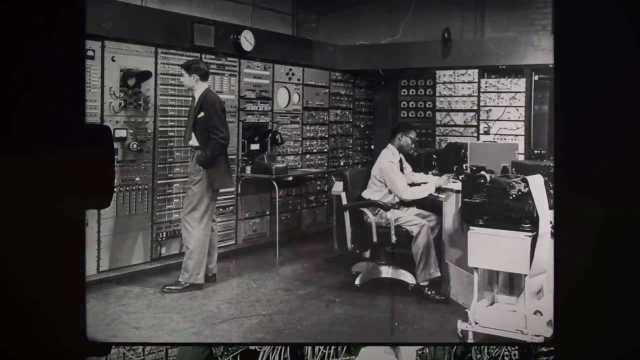 So it was slow And there were lots of areas that we just couldn't explore because it was beyond our computational ability. But then we developed early computers And that allowed us to input larger data sets and answer problems that had previously been out of reach. 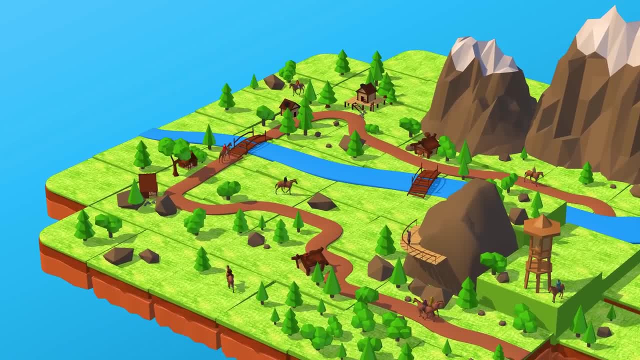 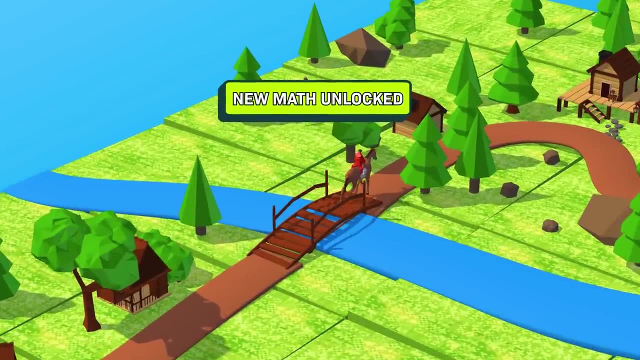 These new computers unlocked new areas on our mathematical map. Instead of walking everywhere, we can now ride horses, We can get farther faster And we can access areas that were previously inaccessible. But there were still parts of the map that our computers couldn't access. 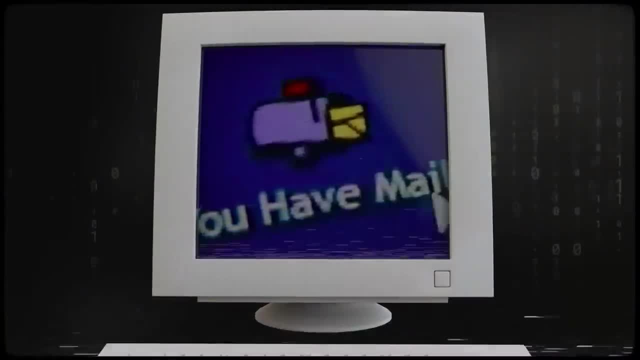 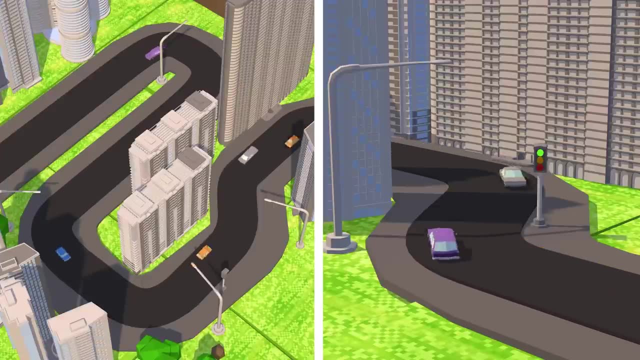 Luckily, computers just kept getting better, And they allowed us to solve more and more complex math problems. As a result, our virtual map has transformed. We have roads and cars, And we're just reaching areas that were previously unreachable. Better computers mean traveling across this map faster. 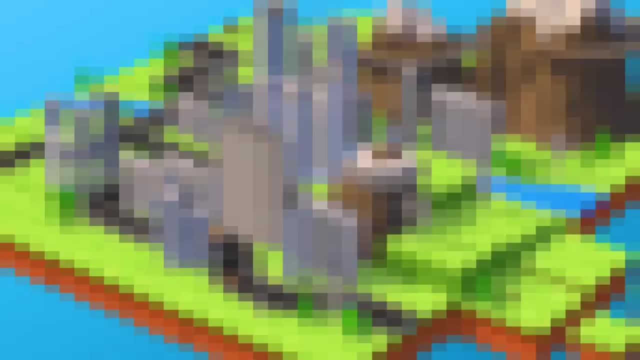 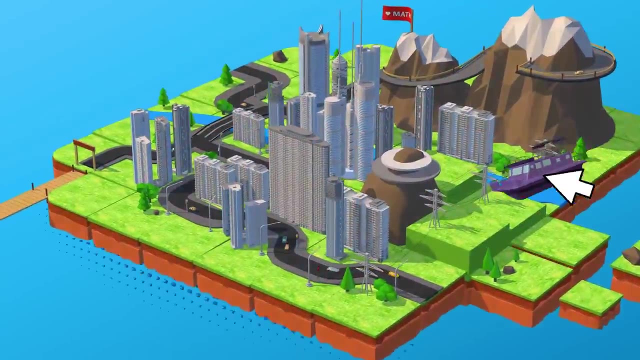 and more easily than ever. The thing that he said was really important to understand is that quantum computers are not faster cars, They're boats. A boat is not necessarily better than a car, They're just built for totally different terrain. So with our new quantum computers, 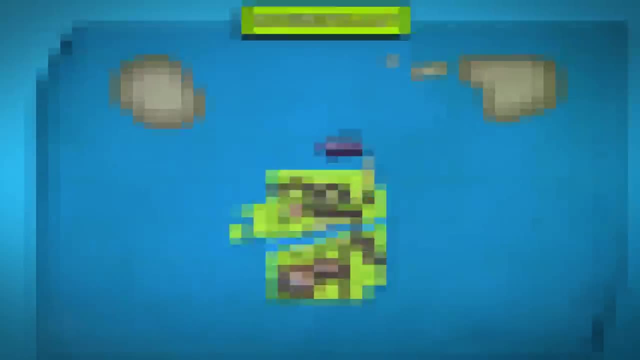 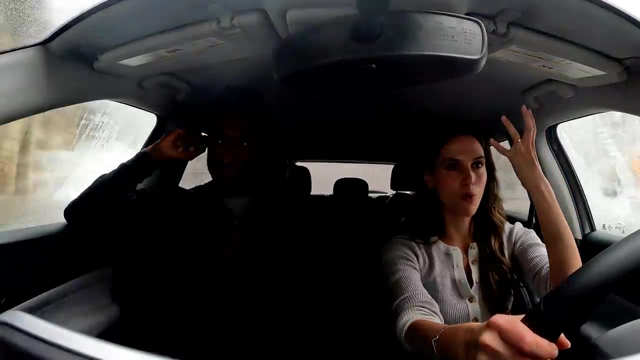 we're beginning to navigate These new mathematical waters, Solving problems and discovering areas that traditional computers just can't. My question for IBM is: what's in the water? Oh wow, What are the oceans that we're all of a sudden? 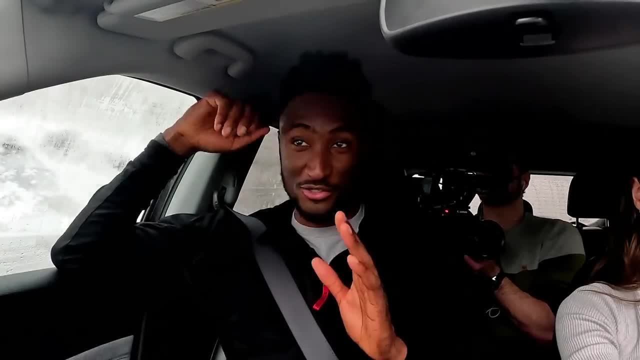 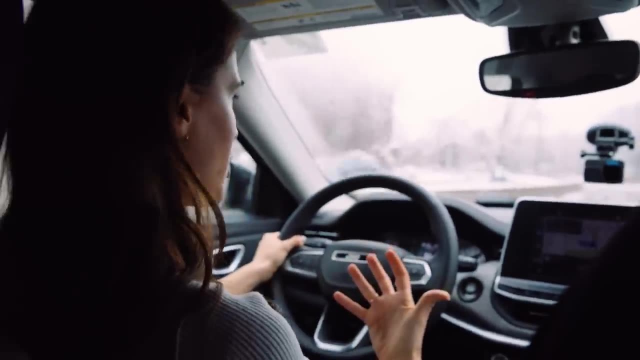 able to explore with our quantum computer boats. I love this. I'm an analogy person, so I'm fully absorbed in this now. This is why I think a quantum computer is never going to beat an iPhone, But I think that this is a better thing to offer the audience. 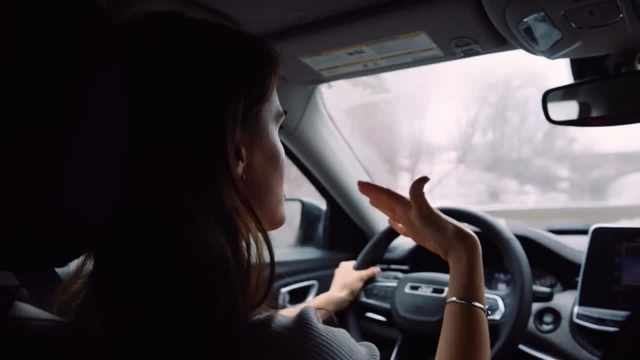 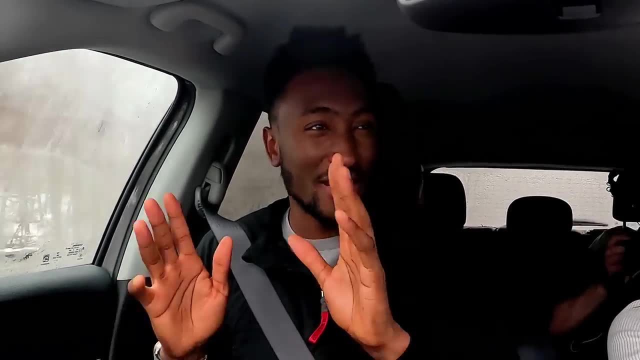 It's a better offer, you guys, instead of quantum computers are just another exciting computer. I guess what people are probably clicking on this video thinking in their head is: will there really never, ever be a quantum computer in my pocket? And I guess that would be. will there ever? 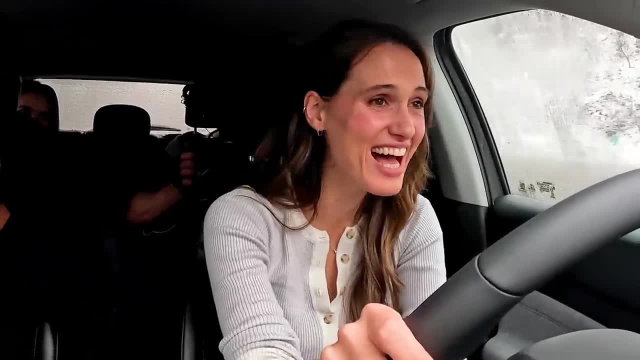 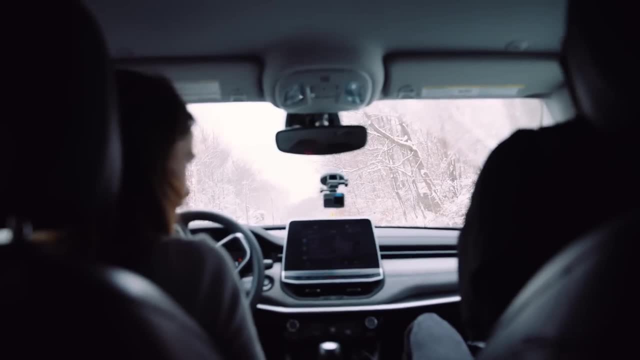 be a flying car boat. you know, Is the tech ever going to get to that point? Just a question. I just want to say I really appreciate your commitment to this analogy. I love it. I love the analogy. Guys, we have arrived. 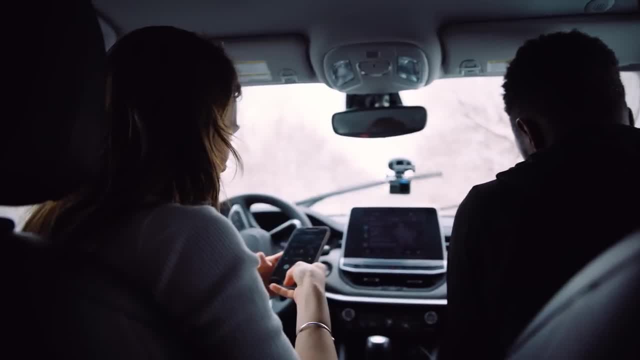 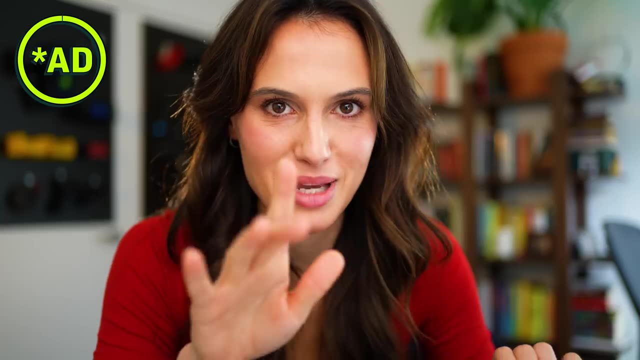 Where have we have arrived to? This does not look like there's a quantum computer here, IBM Research Division. Here we go. OK, before we get to IBM, I want to show you something. So I travel a lot for Huge, If True, episodes. 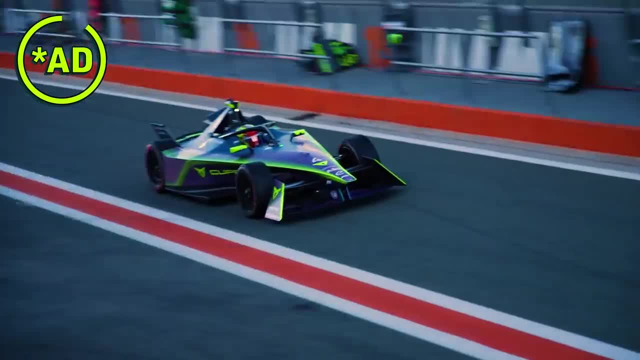 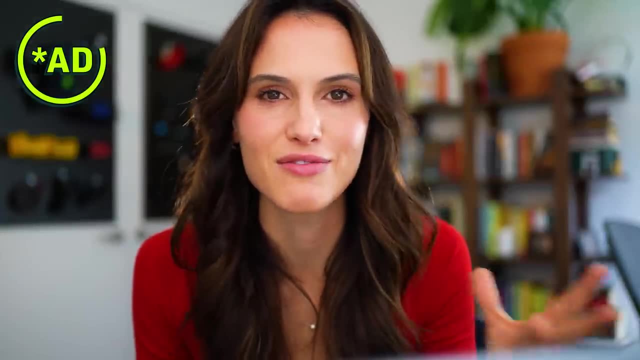 I went to Spain recently to visit behind the scenes at Formula E testing, which was really, really fun. But often when I travel I want to make my computer believe that I'm still in the United States, just so that everything online feels normal to me. 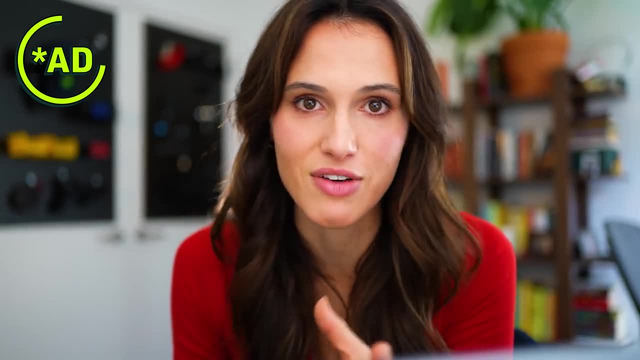 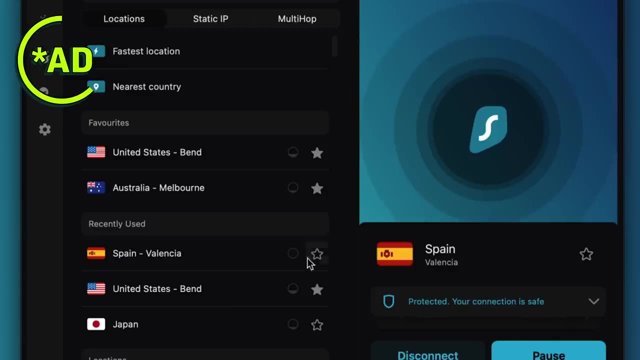 The websites that I visit are in dollars. The TV shows that I like never get blocked, that kind of thing. The way to do that is with a virtual private network or VPN, Specifically this one, Surfshark. If I'm using Surfshark and I set it to the United States, 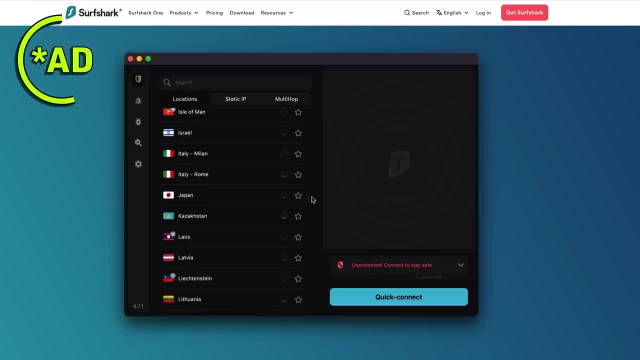 I can be at home online even when I'm traveling, which is really nice, But sometimes I want the opposite. I want my computer to think that I'm somewhere else when I'm actually at home. You might not realize that a lot of things. 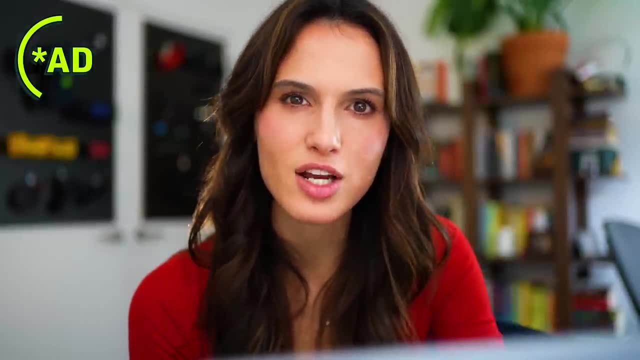 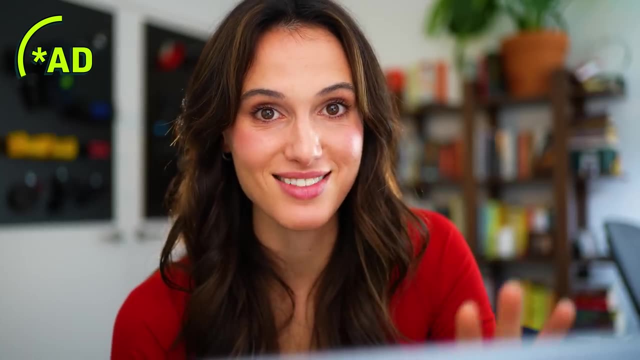 like, airline flights especially, are priced differently depending on where they think you are when you're buying them, Which, but also you don't have to put up with that. So when I use Surfshark, I can set my location to one of 100 different countries. 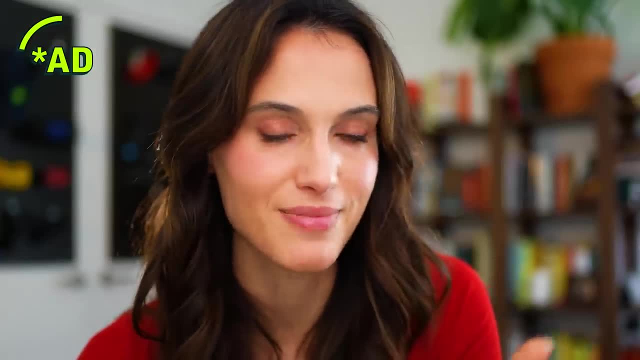 and then hopefully spend less. If you don't already use a VPN, you might find it useful. I know I do. If you want to try it out, click the link in my description and use the code CLEO for 83% off and three months free. 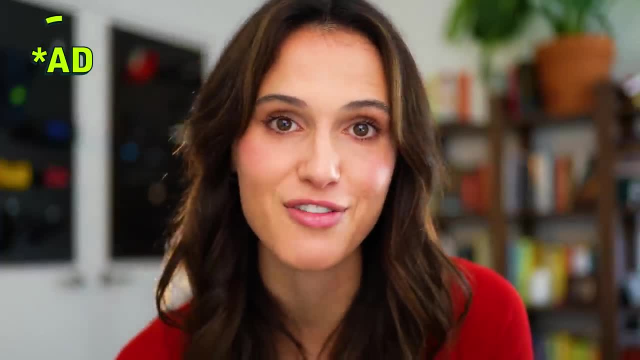 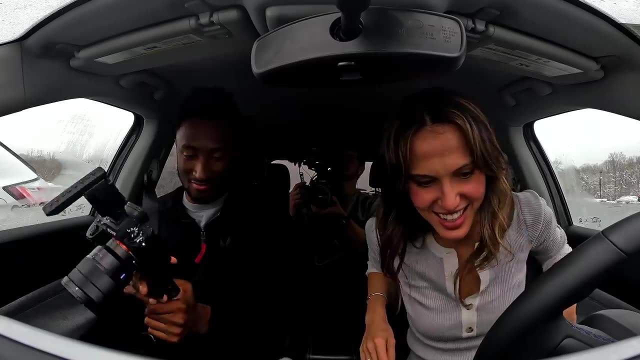 which is just a crazy good deal. I think you'll probably like it, but if you don't, they offer a 30-day money-back guarantee. So go check them out. Now back to the story. All right, Let's go. 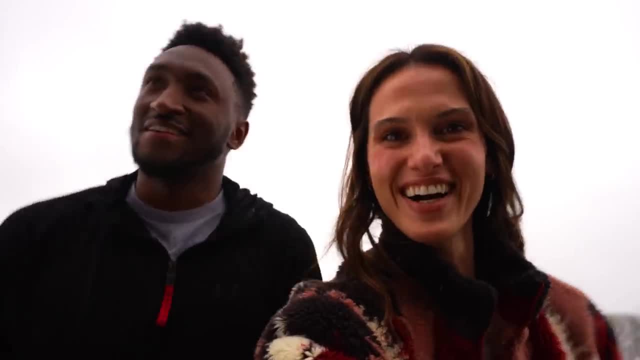 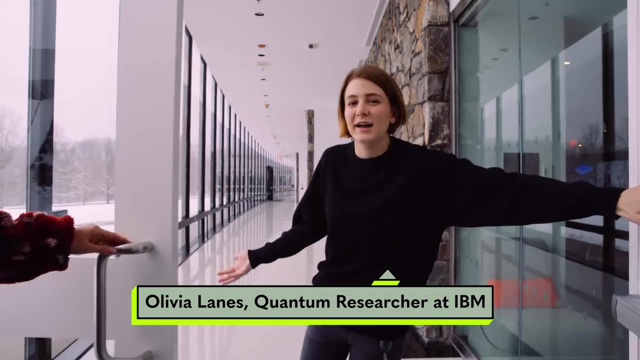 Let's go see a quantum computer. We made it, We're here, Here we go. Do you want to introduce yourself first? Oh sure, Olivia, audience Audience. Olivia, Hi, I'm Olivia Lanes, I'm a researcher at IBM and I also 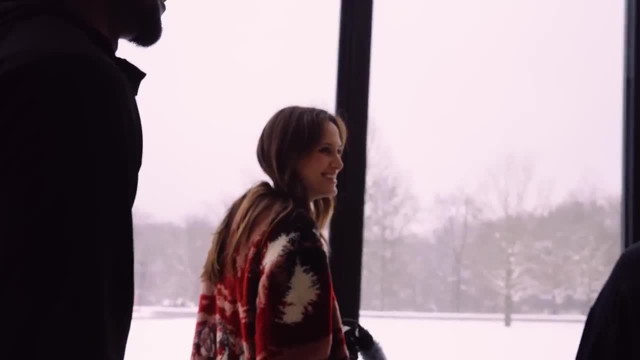 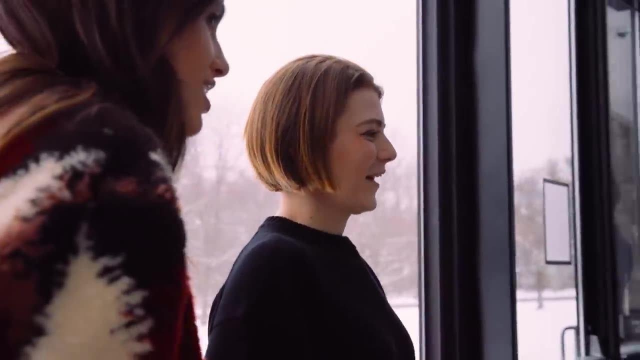 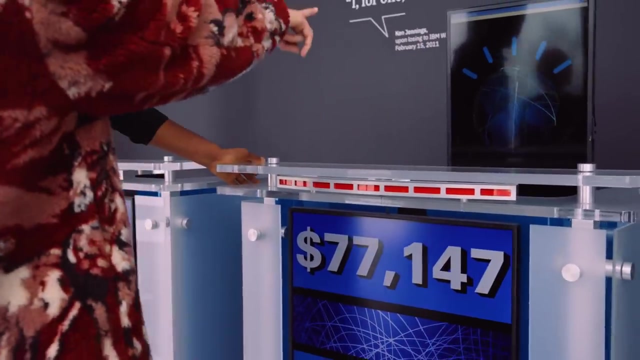 work on the education and the community team, We're going to go look for a quantum computer. What's going on here? This is our Watson setup. No, please go ahead. This is where the Watson AI thing was displayed, and it competed on Jeopardy with Ken Jennings. 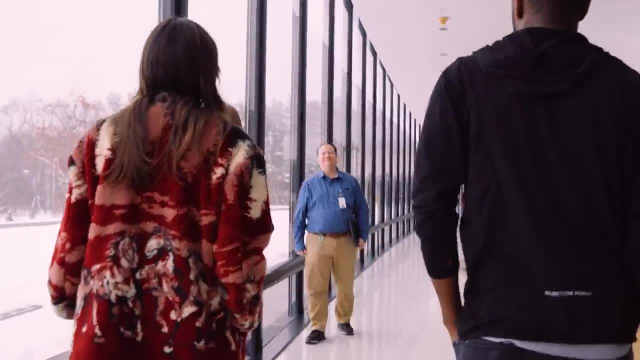 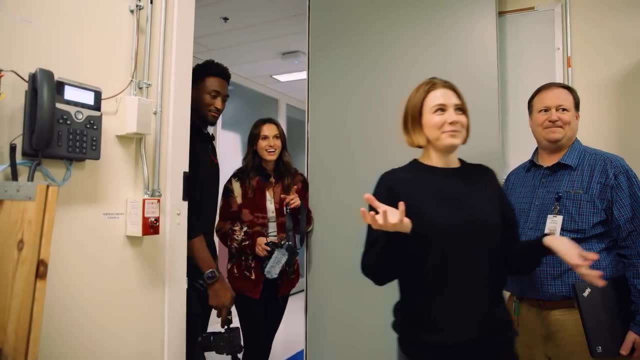 Watson, what is Chu? You are right, This is Brent. It's Brent's lab, so it's very nice of him to let us in. Great to meet you. Thanks for having us. So this is the lab That's the quantum computer. 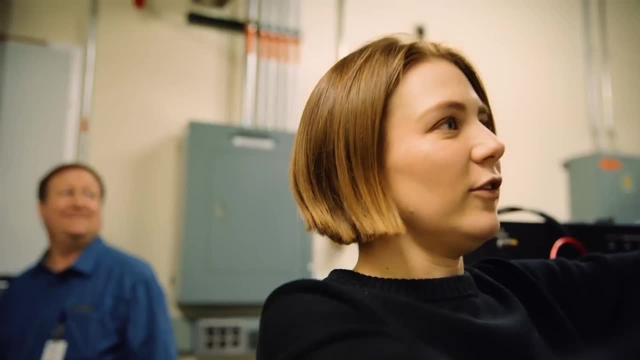 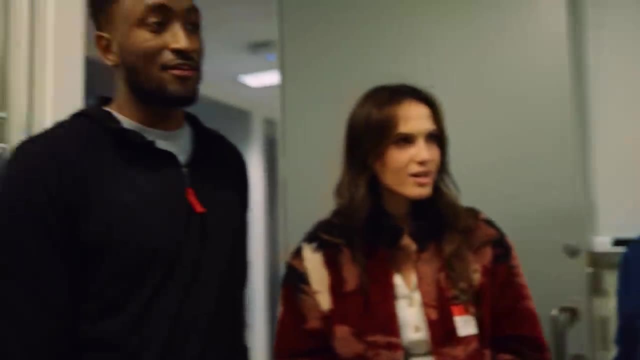 Yeah, Actually this is a dilution refrigerator. This whole thing is basically constructed to keep the quantum computer very, very cold. 15 millikelvin, It's the coldest thing basically in the universe. It's colder than outer space. 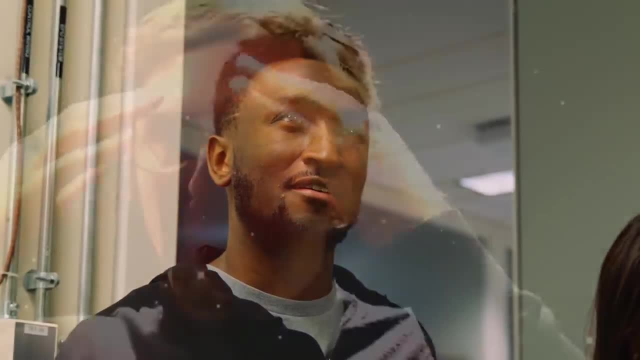 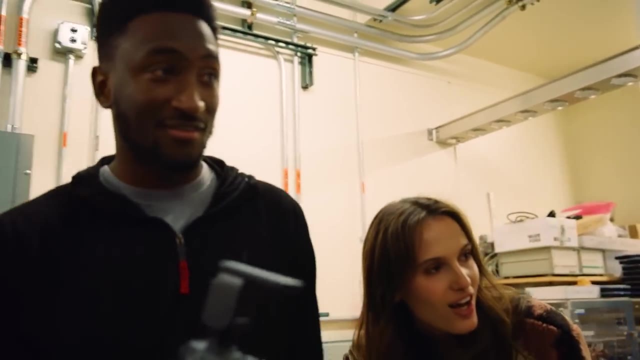 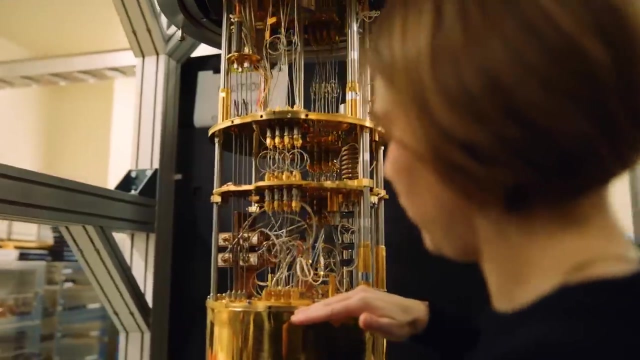 So inside, that is 15 millikelvin, Yep. So here let me show you the one that we can like play with. This is it. This is a quantum computer. This is a quantum computer. The quantum computer is a chip in this one here. 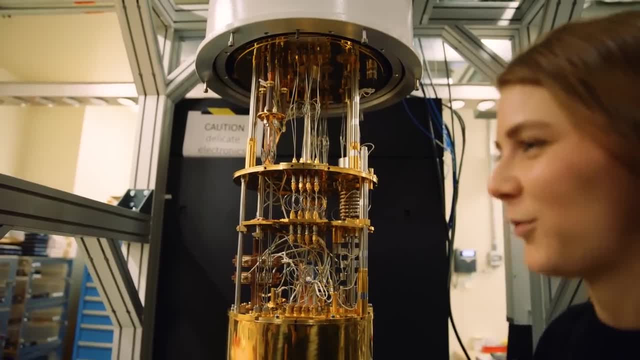 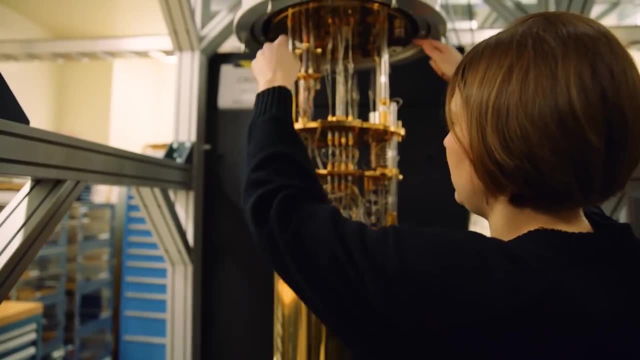 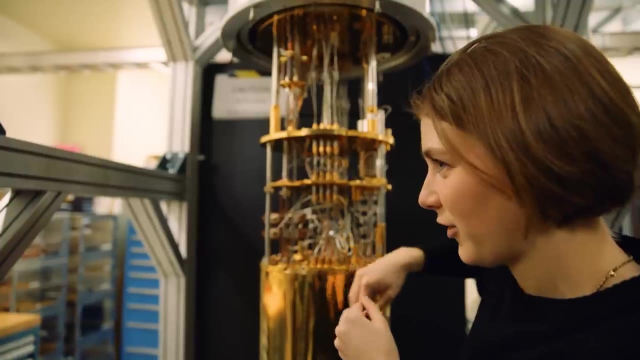 But this whole thing keeps the quantum computer working at insanely cold temperatures, like we talked about. So this is all refrigerator technology, So all of these cables that you see here on the side carry signals Down through the fridge into the processor and then they do their quantum stuff. 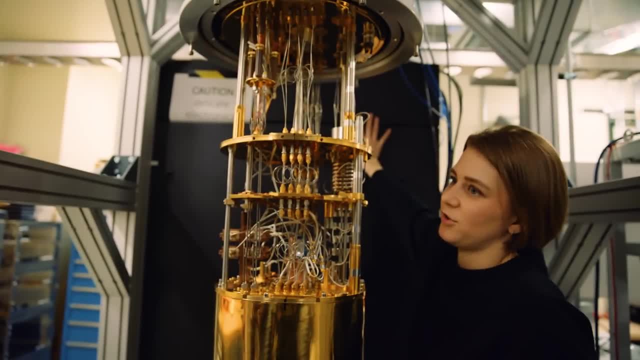 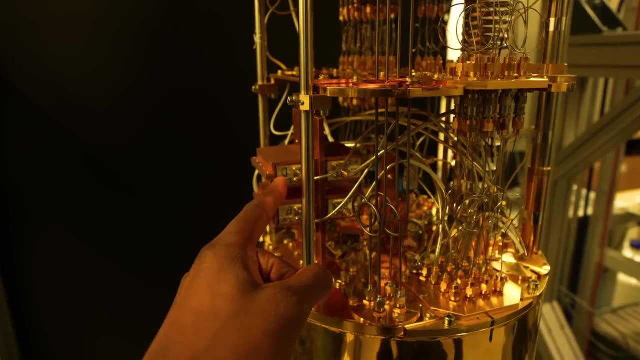 And it comes up And it goes to these room temperature control electronics And they turn it into things that humans can understand. That is a quantum computer. We were allowed to touch it, which was cool, Oh my god. So I think it's really funny that when people generally 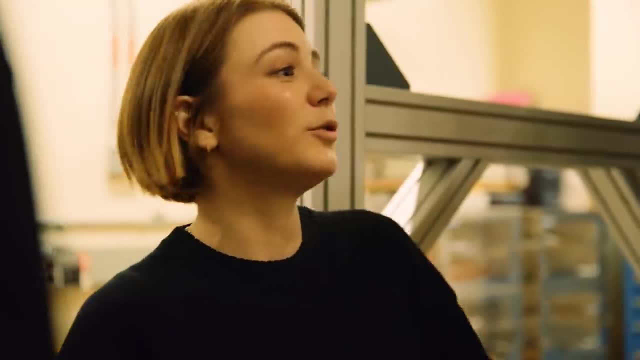 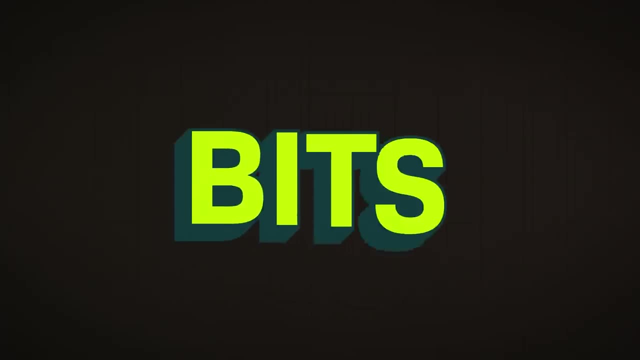 talk about, like the difference between classical and quantum computers. people are like, OK, well, you know how a classical computer works, right, But like the truth is that, like nobody knows that Simplification, Simplification of it is, it comes down to bits. 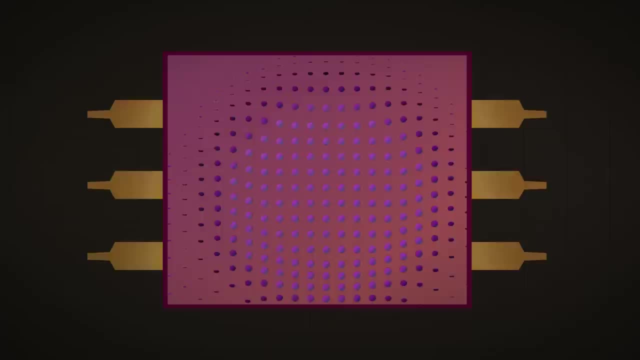 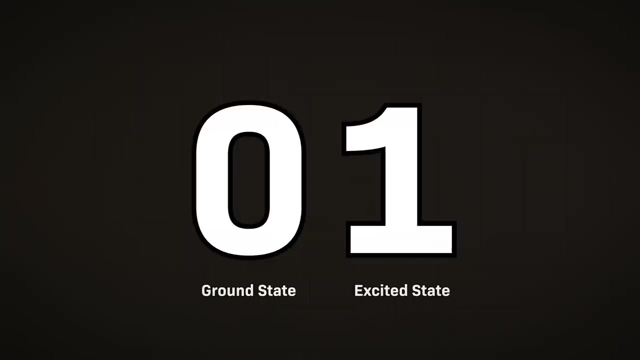 And bits are made out of pieces of silicon And you have, you know, tens of thousands to millions of them in your computer And they can either be in the state zero or one We call it the ground state or the excited state. 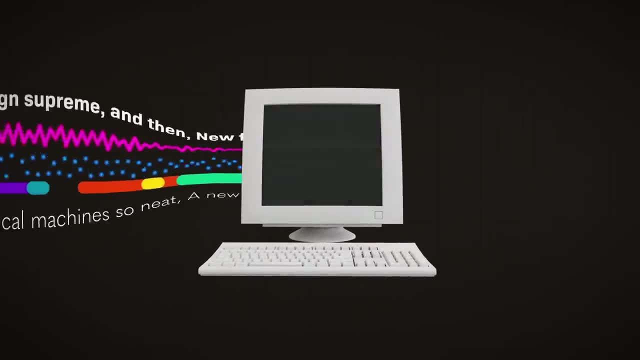 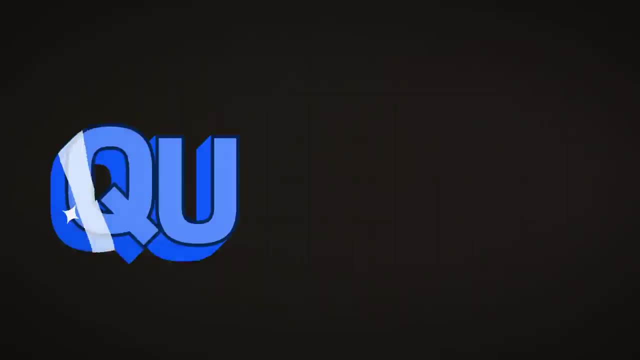 And everything that you type into your computer, like all words, all numbers, all colors, get translated into computer speech. But it's very binary, right? A quantum computer is run on qubits. Cubits aren't like bits, They aren't a one or a zero. They're more complex. Think of this like a wave. A qubit could be really likely to be zero, which means a lower energy wave, Or it could be really likely to be one, which means a higher energy wave, And each qubit has a probability of being each. 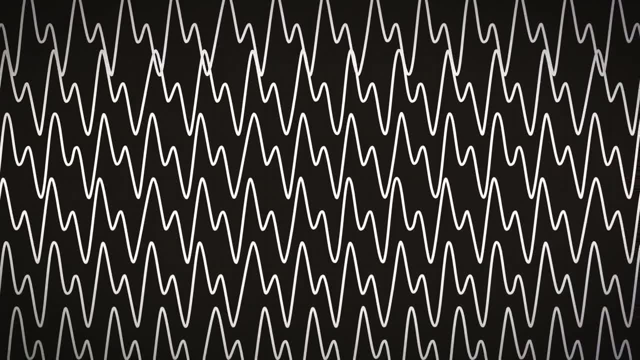 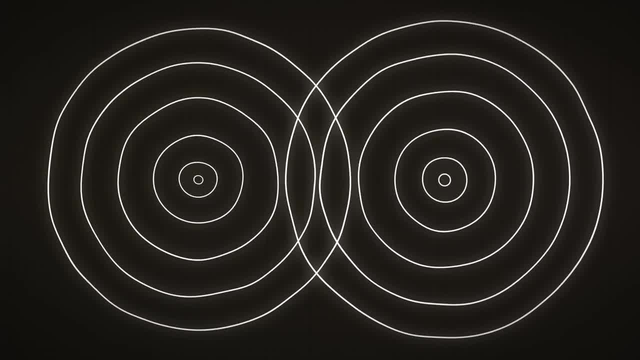 When a quantum computer is working, the probabilities of multiple qubits interact And they add constructively or destructively, just like waves would, If you were to like, tap like two places in a pond. You know how, when you like, explain something. 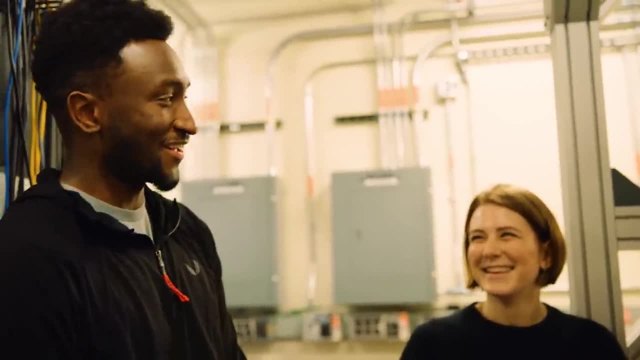 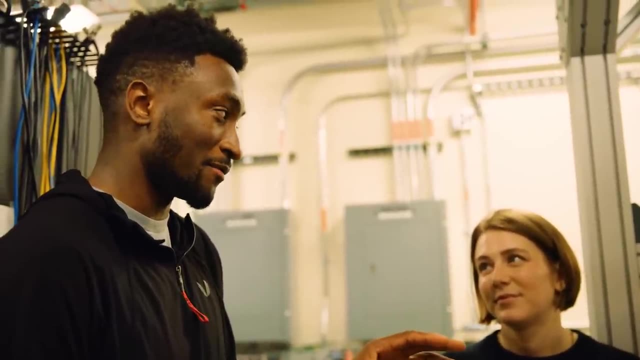 to a two-year-old and they just keep going, oh, And you're like why? And they have to explain it again and you go: why? Yeah, My question is: as the controller of the computer, you decide. what about those probabilities? 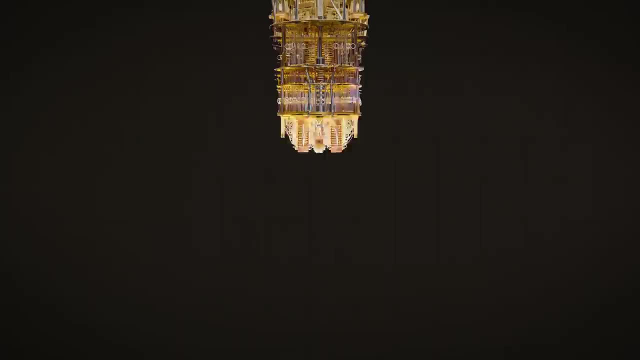 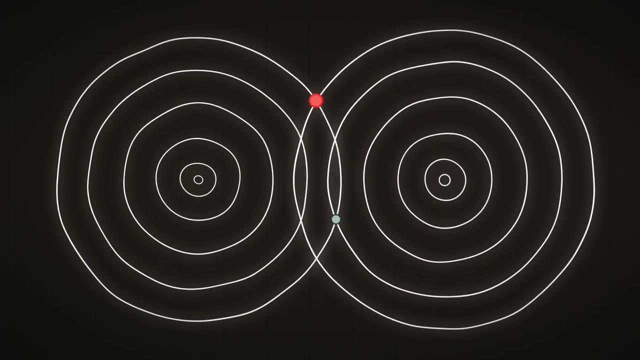 Basically you are altering the probabilities while you're running an algorithm. It's a common misconception that quantum computers try all the options. That's not right. This is simplified but it's more like a quantum computer kind of watches the pond. It watches how all of those waves interact. 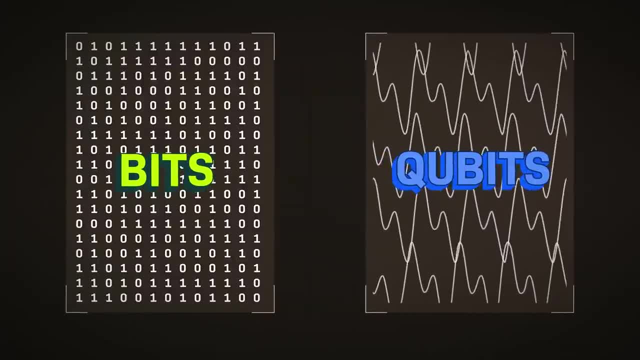 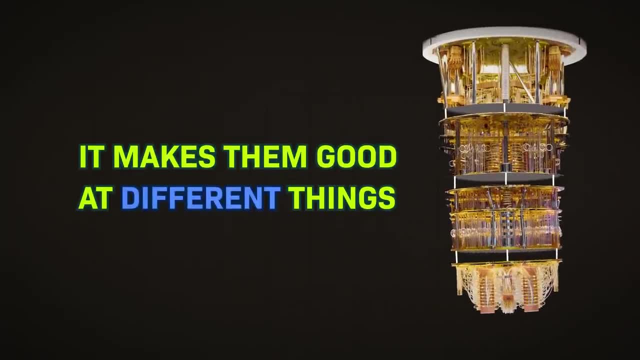 and then finds the most likely answer. If this is all confusing, don't worry. All you really need to know is that quantum computers calculate things very differently than classical computers do, And that makes them good at different things. Quantum computers are not going to be faster at everything. 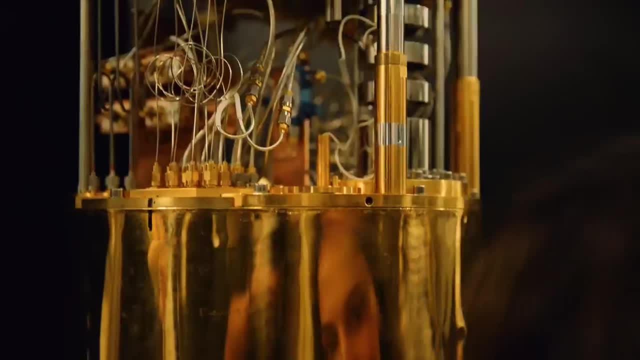 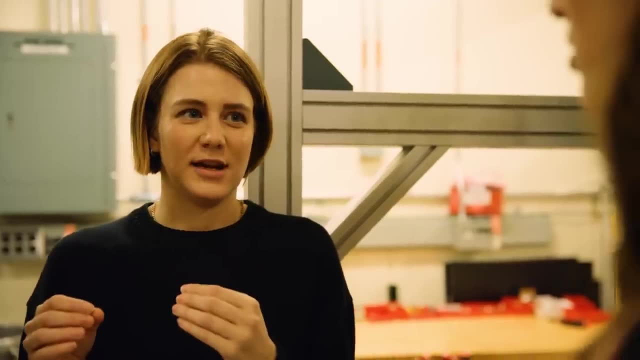 than a classical computer. Like it's not good for addition, right, Because your calculator and your phone is perfectly good at that. But the things that quantum computers are good at is finding structure in tons of data And if you're interested, we can close it back up. 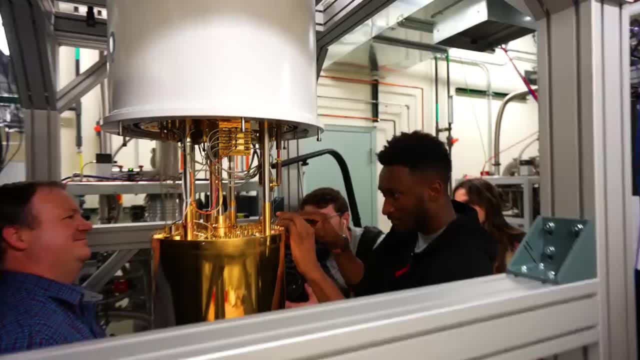 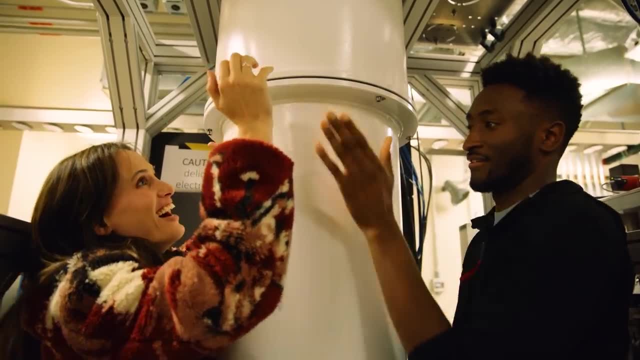 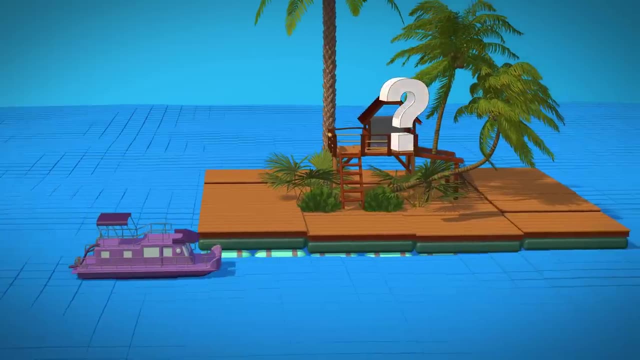 Absolutely Put us to work. Yeah, Let's go back to our virtual map. So we have our boats and we're floating around discovering new parts of this map. One of the first new areas of interest is simulating nature. Simulation of nature seems really interesting. 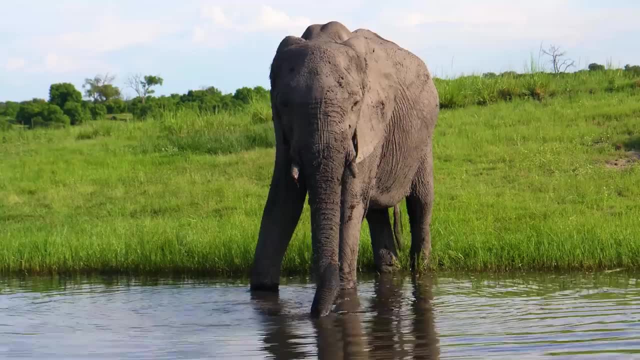 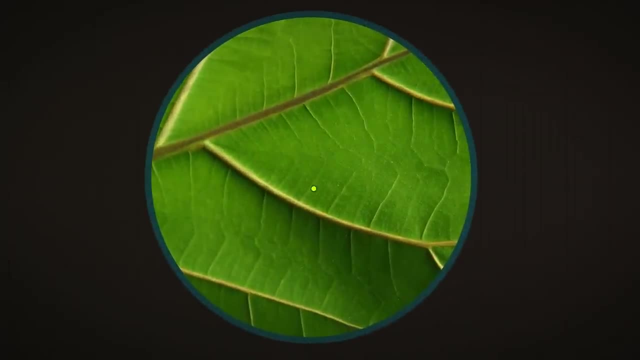 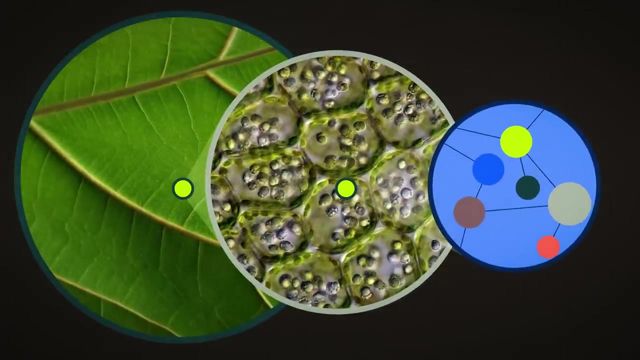 Why is nature one of the things? So nature fundamentally is quantum and it obeys quantum physics. We just don't want it, don't normally see it, but if you look at a molecular level and the atomic structure of molecules, everything has to follow the laws of quantum physics. 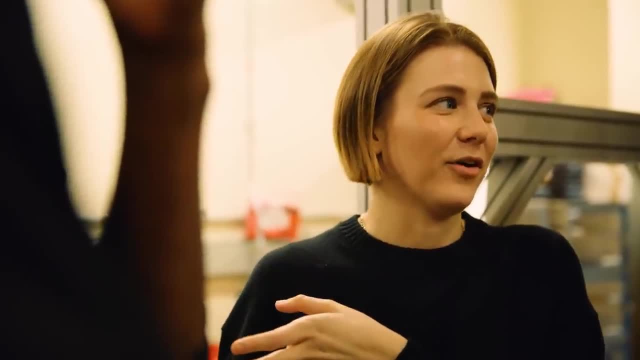 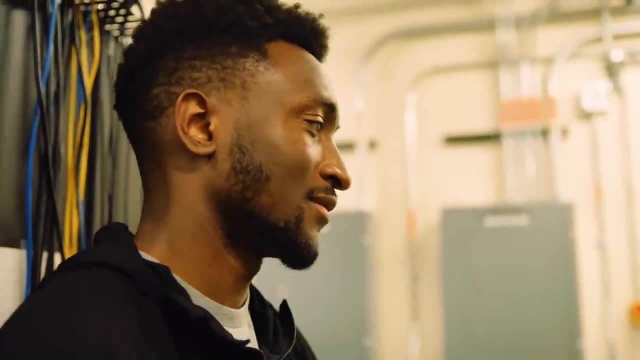 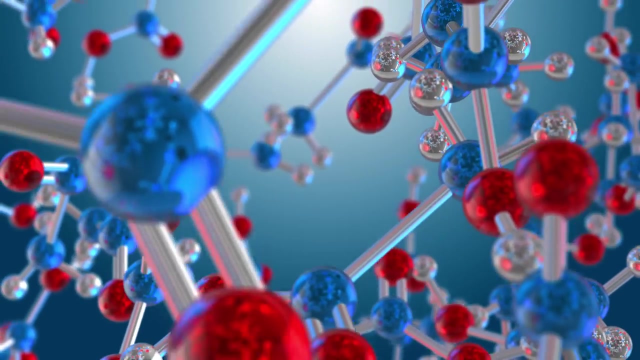 It's really hard to calculate what a material or what an atom is going to do past a certain size. So at a certain point it just can't do it. But if you're interested in developing battery technology or creating new materials that have long chains of molecules, you're going to need a quantum computer. 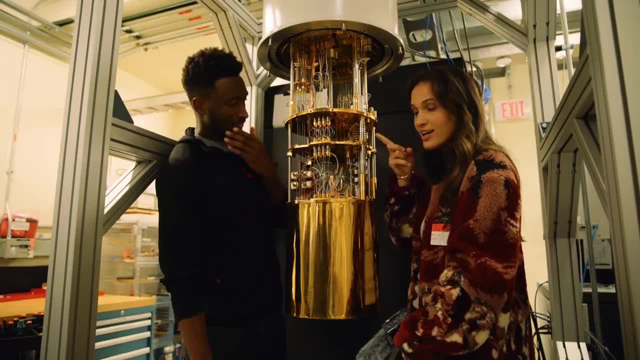 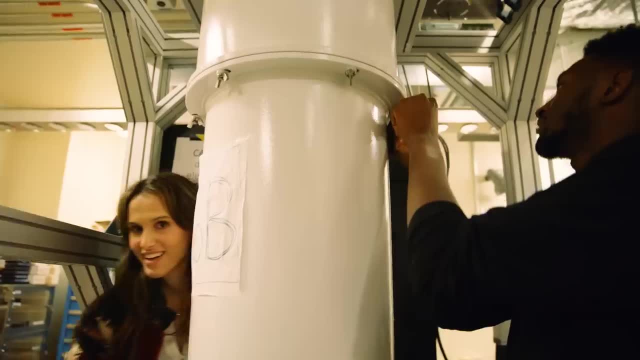 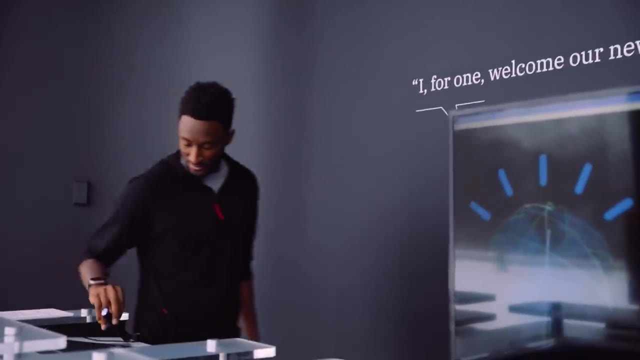 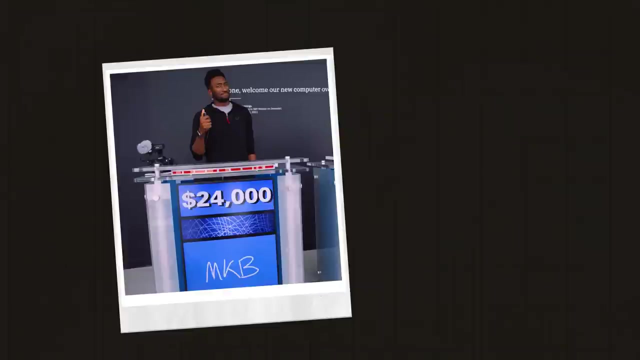 This is why people are so excited. Think of the new materials or medicines or molecules that we could make if we could better predict the way that nature behaves at a molecular scale. Oh yeah, Yeah, There you go. Boom, Boom, Boom. 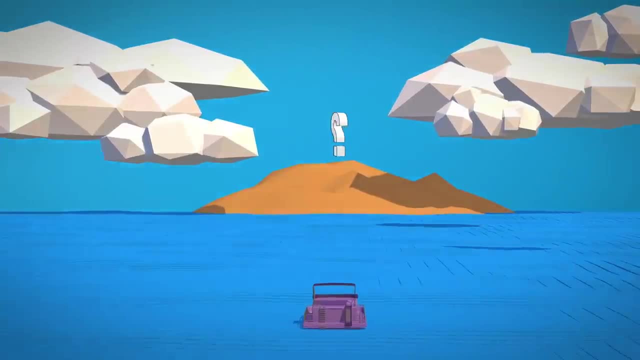 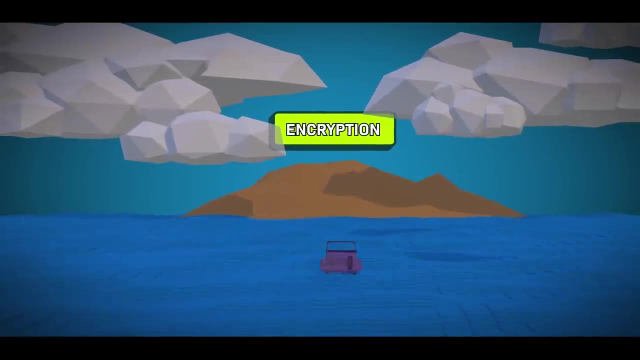 Okay. so simulating nature is something that quantum computers could be amazing at, But we're also getting closer to another use for quantum computing, one that people and governments are more concerned about: Completely new encryption algorithms: Break encryption, Quantum-resistant encryption. 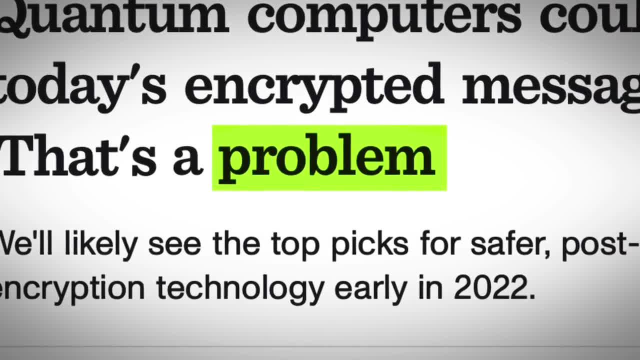 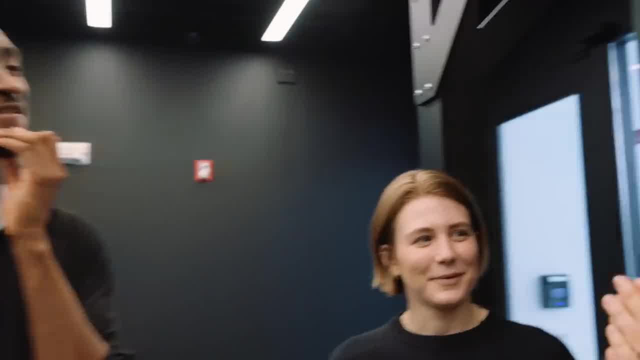 A fully functional quantum computer could be built with code-breaking capabilities that could render all forms of online encryption unreliable. Okay, now, this is the one that I've been waiting to ask about. Why is everybody so obsessed with talking about quantum computers and encryption? So the first major algorithm that was developed for quantum computers is Shor's algorithm, named after Peter Shor, super nice guy. He invented an algorithm which basically can find factors, prime factors for really large numbers. Why does anyone care about this? 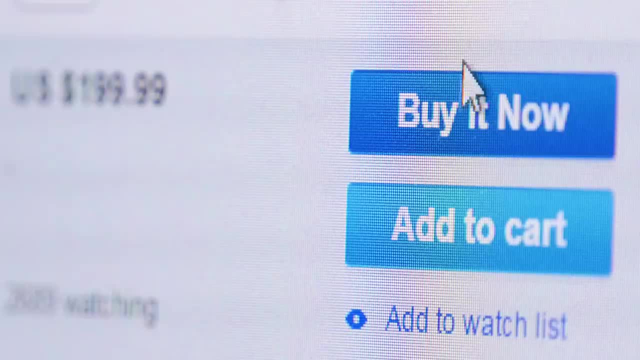 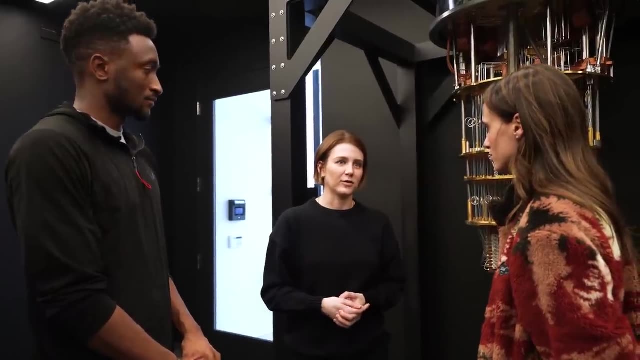 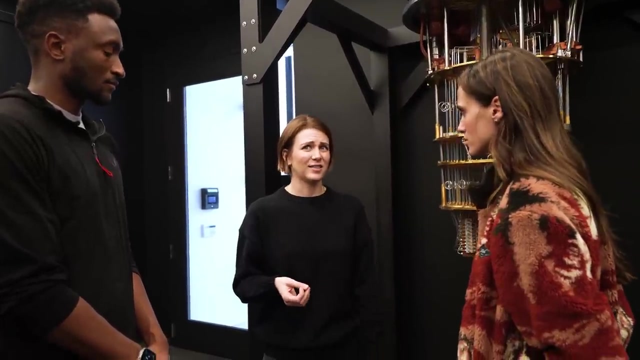 Because that's the basis for RSA encryption, which is basically how all transactions on the internet are conducted. The entire reason that all of our encryption schemes today work that way is because it's basically impossible to crack that with a brute force. classical algorithm It would take, I think it's like billions of years. 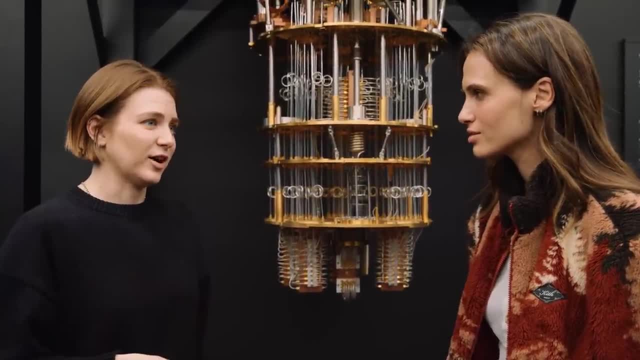 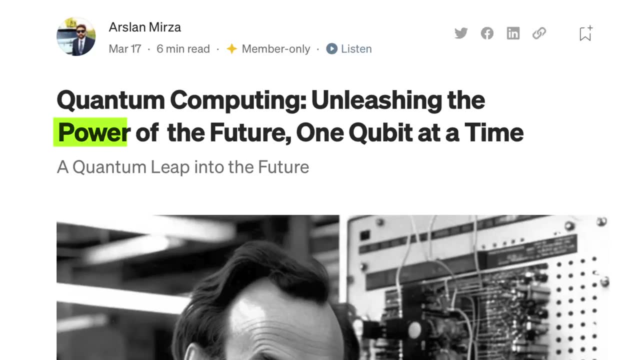 But a quantum computer could do that way more efficiently. We're talking hours to days, So this global race now makes a ton of sense. Whoever gets a quantum computer to actually do this has a big, obvious advantage. But we haven't done that yet. 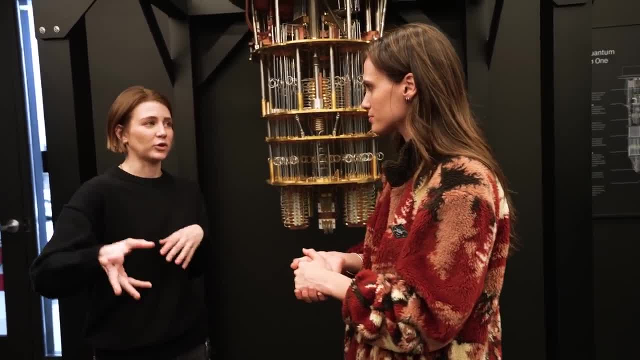 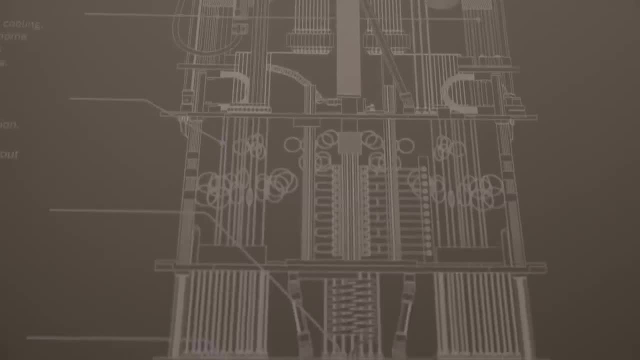 That's one of the ones that requires Okay, Okay, Okay Okay. There's probably like a million qubits or more to do, but we're working up to it. So we're not going to be using quantum computers to break all internet security right now. 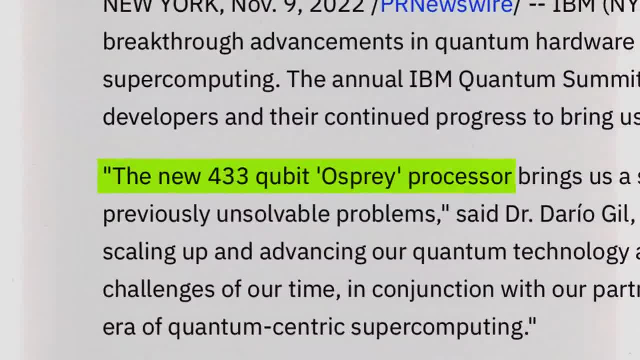 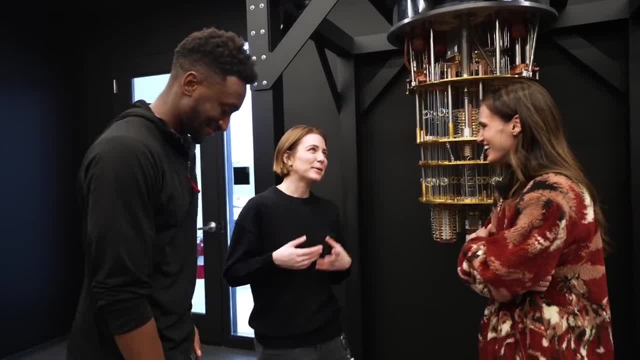 Today we're at 433 qubits, the record set by IBM. Four hundred to a million qubits is a big difference, But Olivia is confident that we'll get there sooner than you think. In the next five or even less years we're going to see people switching over to quantum. 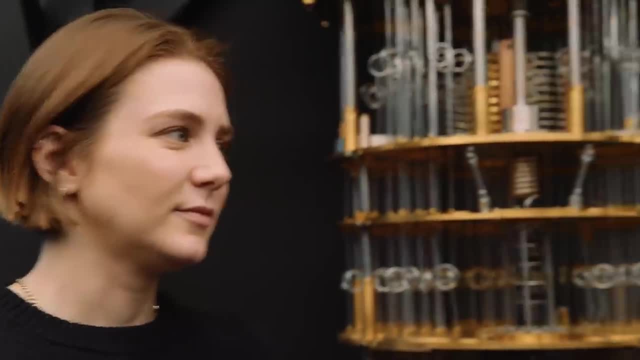 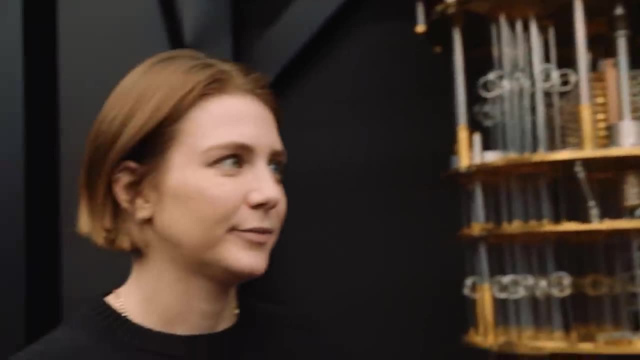 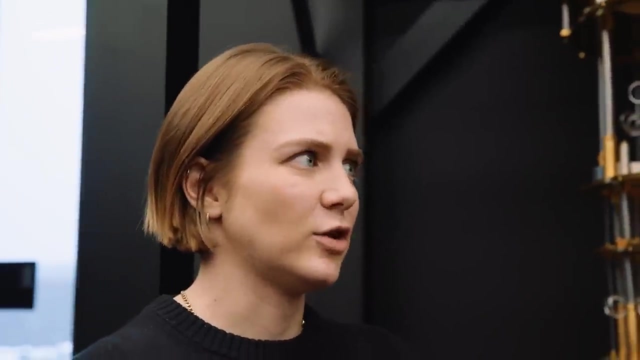 safe algorithms because of this reason. So RSA goes away and we have quantum safe encryption instead. Probably Not all at once, but gradually. you're going to see people do it. We're progressing at an incredibly fast rate. We're solving problems that people didn't even begin to know how to crack two years. 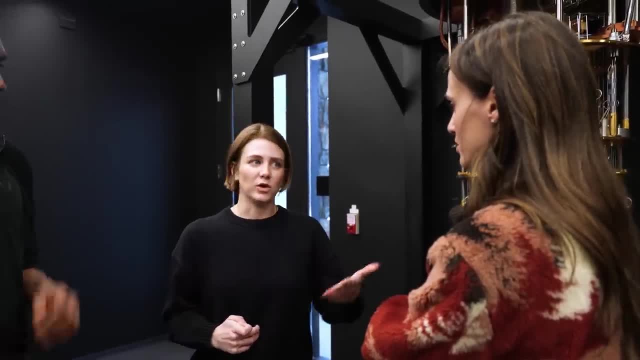 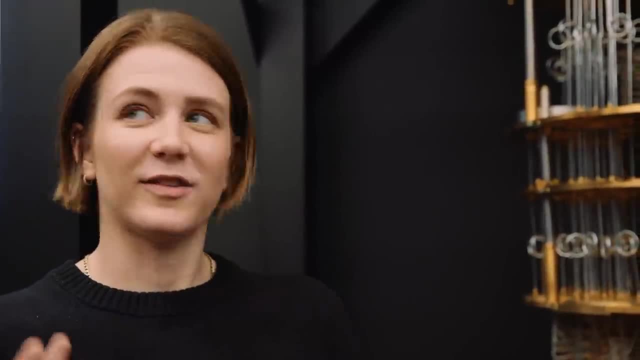 ago, But we've done it Like every single year. everything that we say, we do, we do Nothing mathematically or physically prevents it, And so if the physics says it's allowed, the engineers will find a way. That's sick. 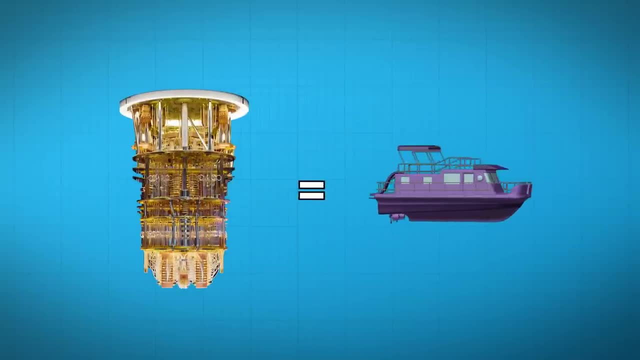 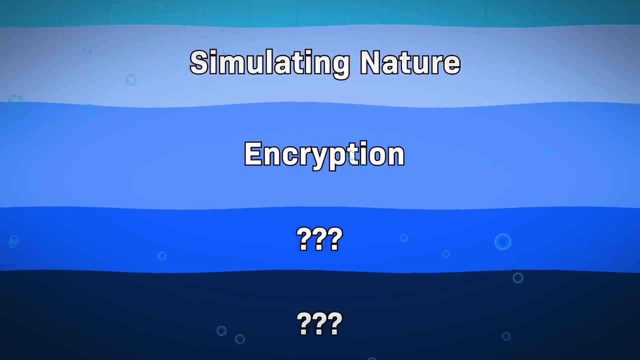 I'm picturing that- I'm adjusting the analogy slightly- that it's submarine because there are sort of different levels of quantum computing. Yeah, we are just skimming the surface. We're going to keep iterating and improving upon this technology every single year. 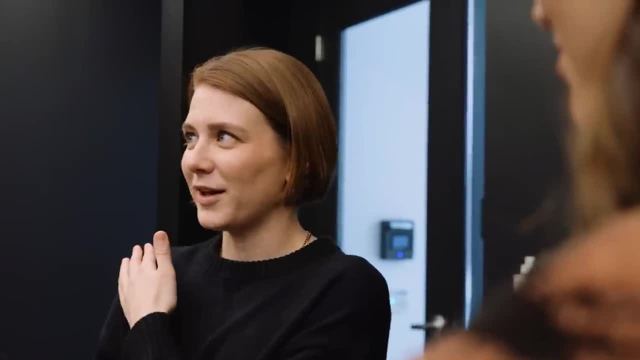 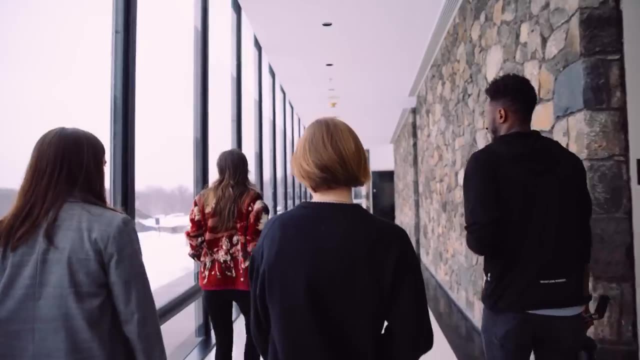 And we're probably going to discover, like new applications, that we haven't even considered yet. It's a bottomless ocean. It's a bottomless ocean. The tour was amazing And as we left we were like, oh, this is awesome. 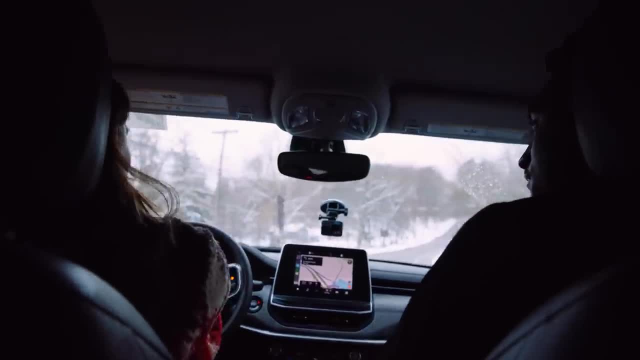 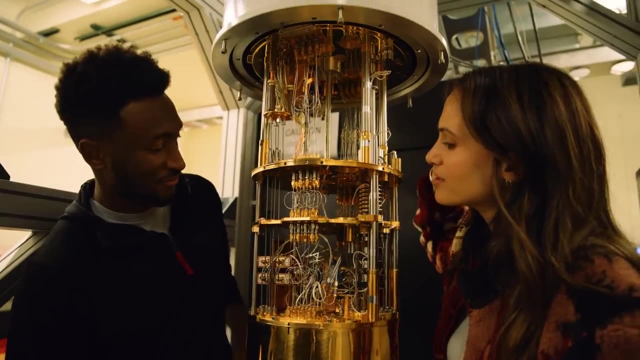 And as we left, we thought about what we learned. Awesome, Let me just get on the highway and then we'll have thoughts. Quantum computers do look exactly like I imagined they look. They look like the pictures, Like the picture, yeah.